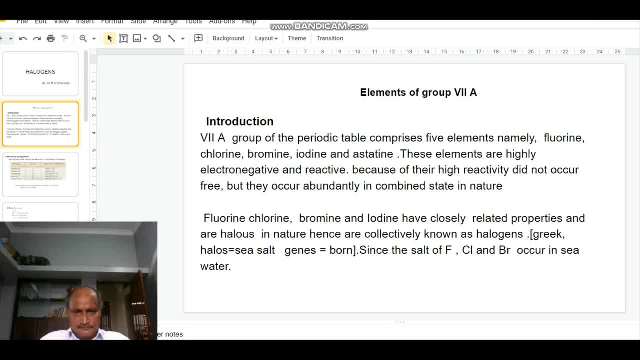 in combined state in nature. Fluorine, chlorine, bromine and iodine have closely related properties and are hairless in nature. hence these are collectively known as halogens. According to Greek, halos means sea salt, zin means born. 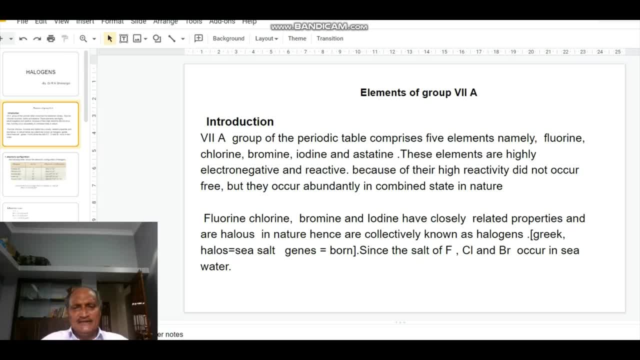 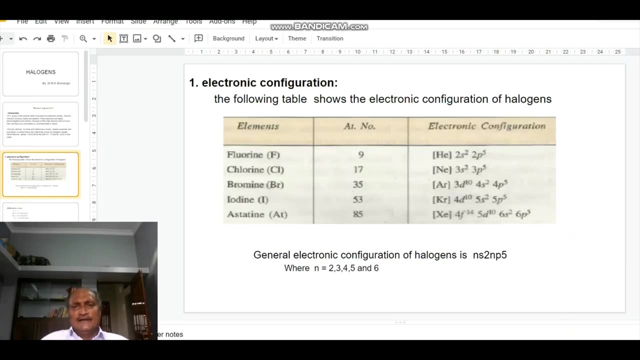 So halogen means a sea-born salt, since the salt of fluorine, chlorine bromine, occurs in seawater. The following table shows the electronic configuration of halogens Elements, their atomic number, their electronic configuration. Fluorine having atomic number 9,, its configuration is 1s2,, 2s2, 2p5.. 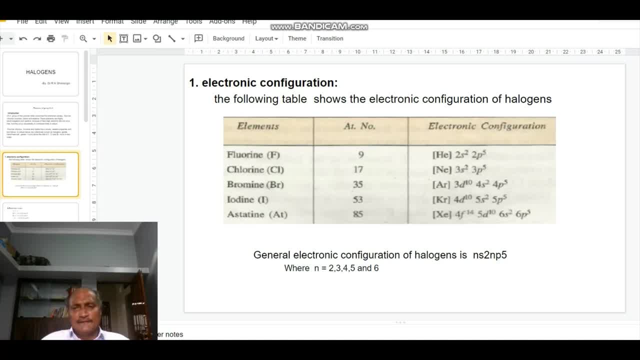 Or 2p2.. After helium, configuration 2s2, 2p5.. Chlorine having atomic number 17, 1s2, 2s2, 2p6,, 3s2, 3p5, or after neon configuration 3s2, 3p5. 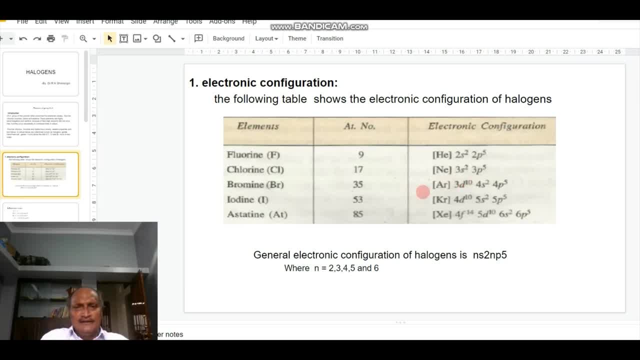 Similarly, bromine, having atomic number 35, its configuration is, after argon, 3d10, 4s2, 4p5.. Similarly, coming to the iodine, having atomic number 53, its configuration is 4s2, 4p5. 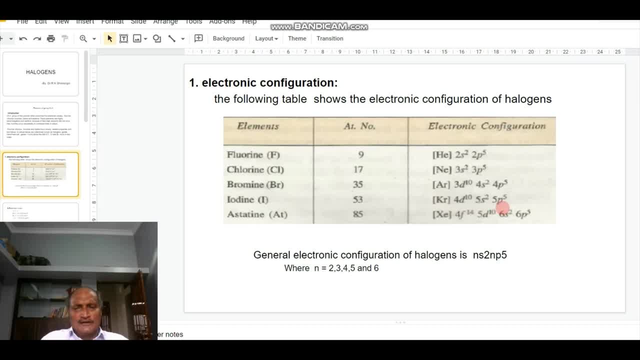 After krypton 4d10,, 5s2, 5p5.. Finally, coming to the last member of the halogen, that is, astatine. symbol is 80, atomic number is 85,. its configuration is: after xenon 4f14. 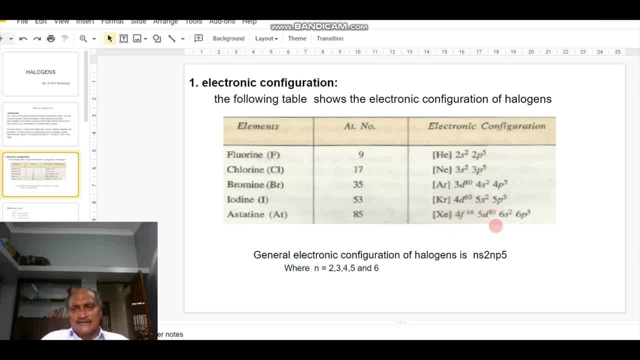 Come on 5d10, 6s2, 6p5.. The table itself indicates the electronic configuration of halogens Generally. here we are going to observe that 2s2, 2p5 in fluorine, 3s2, 3phi in chlorine. 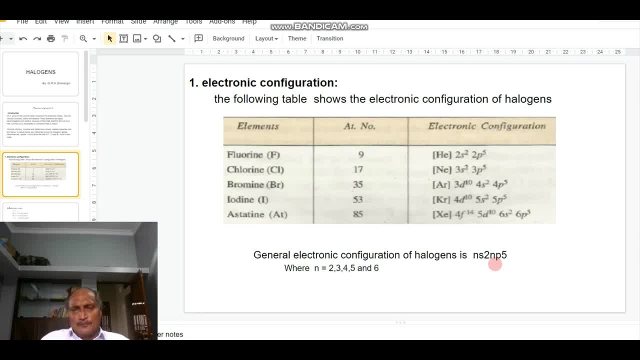 4s2, 2s02, 2h2b. Why we are observing halogens? We are observing halogens 4p5 in bromine, likewise 5s2, 5p5 and 6s2- 6p5 in astatine. 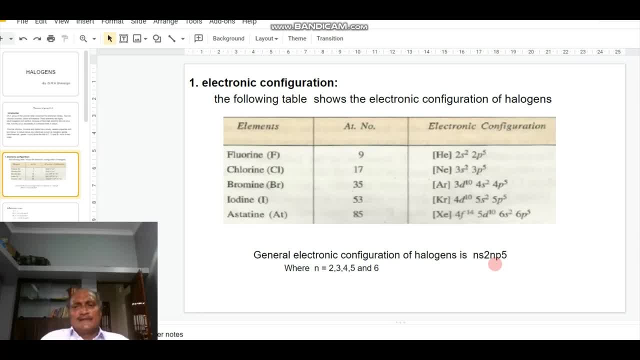 It means the valence cell of halogens contains 7 electrons in the form of ns2np5.. Hence the general electronic configuration of halogen is represented as ns2np5, where n equal to 2,, 3,, 4,, 5 and 6.. 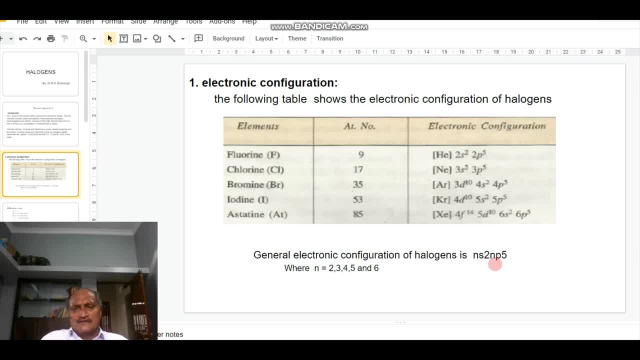 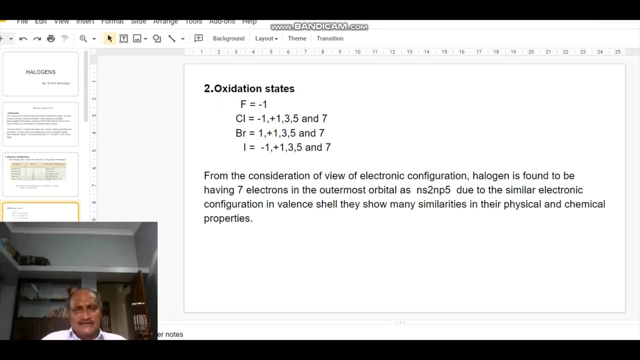 Here the general electronic configuration of halogen is indicated by ns2np5.. Coming to the oxidation states of halogens, here halogen shows number of oxidation states depending upon their ground state and in the various excited states. But fluorine always indicates minus one as its oxidation state, whereas chlorine bromine and iodine indicates, along with minus one plus one, plus three, plus five and plus seven as their oxidation numbers or oxidation states. From the consideration of electronic configuration, halogens is found to be having several electrons in the outermost orbital as nS2, nP5. 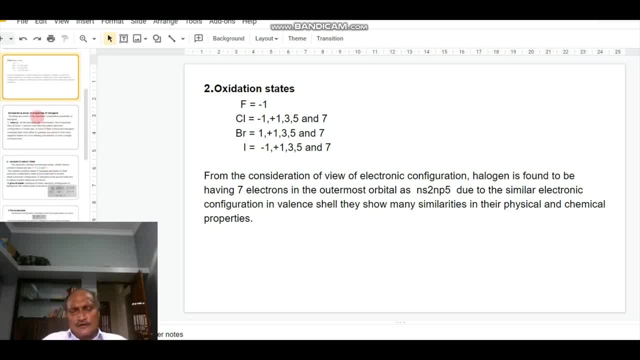 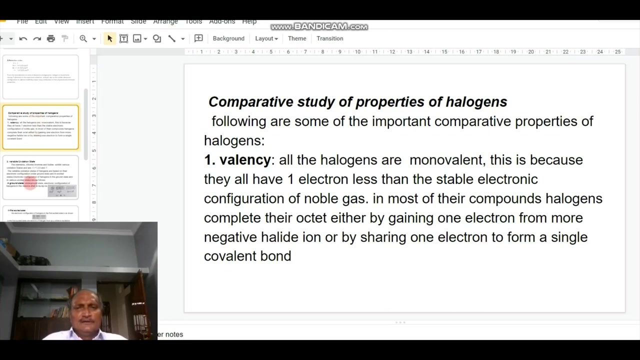 Due to the similar electronic configuration in valence cell, they show many similarities in their physical and chemical properties. So, coming to the properties of halogens, The followings are the some of the important properties of halogens: Valency- Coming to the valency all the halogens are: monovalent. This is because they all have one electron less than the stable configuration of noble gas. In most of their compounds, halogens complete their octet either by gaining one electron from more negative halodions or by sharing one electron to form a single covalent bond. 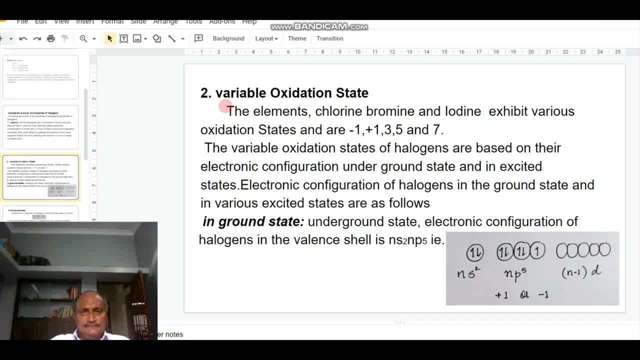 Coming to the second property, ie variable oxidation state, which is an important aspect of halogen, The elements chlorine, bromine and iodine exhibit various oxidation states, and these oxidation states are from minus one plus one, plus three plus five and plus seven. 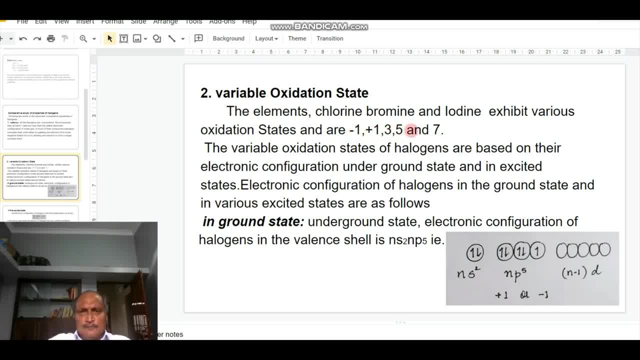 The elements such as chlorine, bromine and iodine are considered to be an important part of the halogen. Bromine and iodine exhibit a variable oxidation state from minus 1 to plus 7,, whereas the element fluorine, the first member, which is a highly electronegative element, indicates. 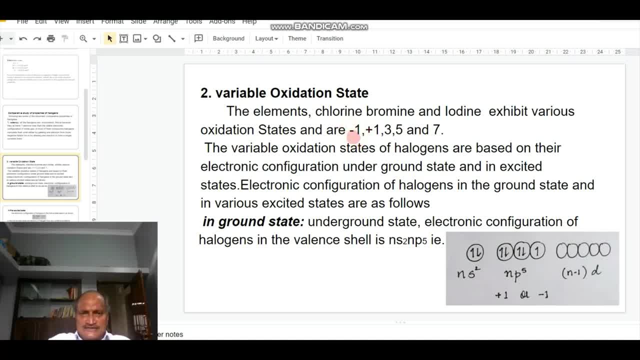 only a minus 1 as its oxidation state or valency. remaining. all elements like fluorine, bromine and iodine exhibit minus 1 to plus 7 as their oxidation states. The variable oxidation states of halogens are based on their electronic configuration under. 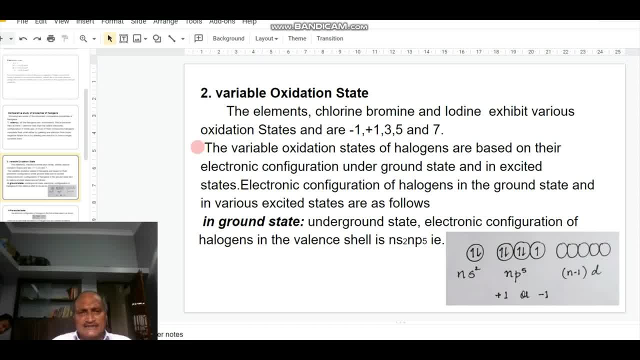 ground state and in various excited states. Electronic configuration of halogens are based on the first element. fluorine and iodine in ground state and in various excited state are as follows: Coming to the ground state configuration: Under ground state, electronic configuration of halogen in the valence cell can be represented: 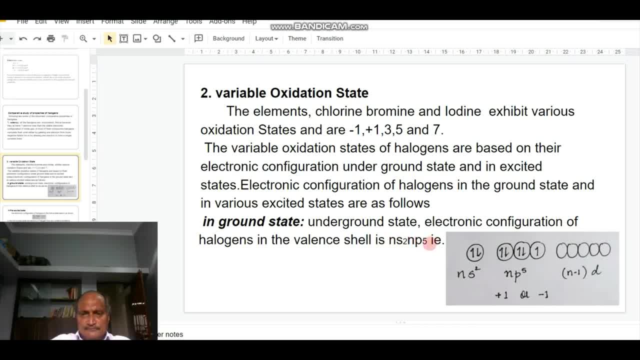 as Ns2Np5.. As we have seen from the electronic configuration, the general electronic configuration of halogens is found to be Ns2Np5.. That is number of electrons present in the valence cell. Totally there are 7 electrons: 2 in the form of Ns2 and 5 in the form of 5p5. 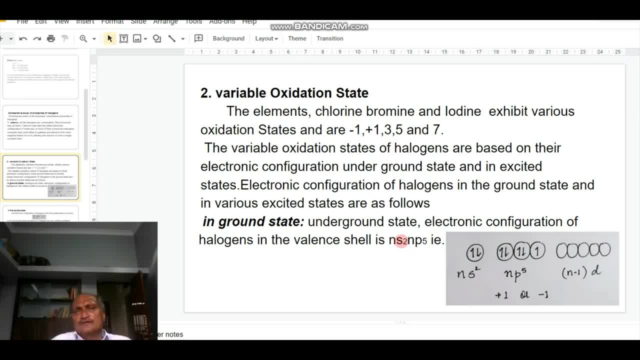 In 5p5, again these electrons are distributed into 5p5.. So this means mantra and demi and neu are available somewhere. 1. Minus two electrons in the py- orbital. 2. Two electrons in pi- orbital. 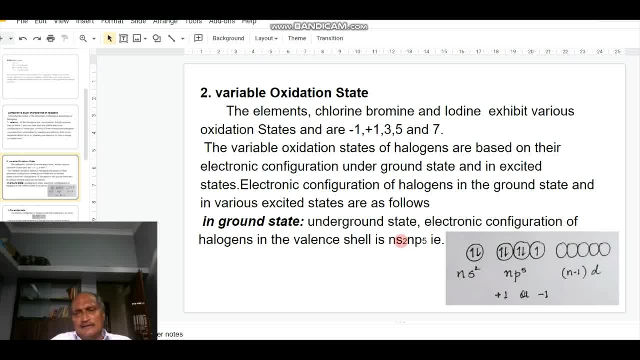 3. Two electrons in pi- orbital, 4. Two electrons in py- orbital, 5. Two electrons in py- orbital, 5. Two electrons in 5py- orbital, 6. Two electrons in 5py, and here this indicates the valence cell configuration of the halogens. 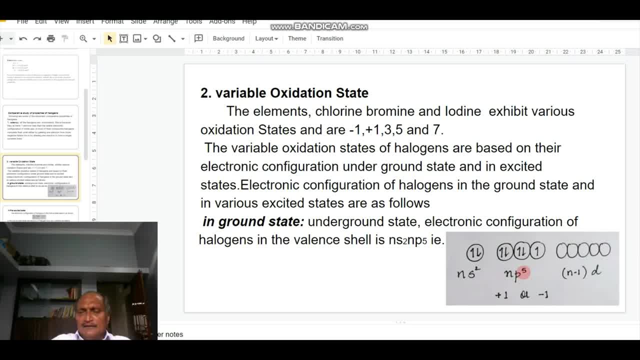 That is Ns2Np5 and no energy concentration, 7. Aa And no energy concentration, and so on. 8. no electrons in the orbital under the ground state of the halogens. hence, here in the ground state, the halogen satisfies their valency either by taking one electron or by sharing. 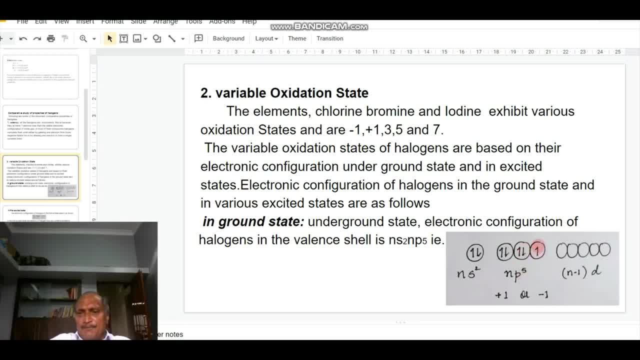 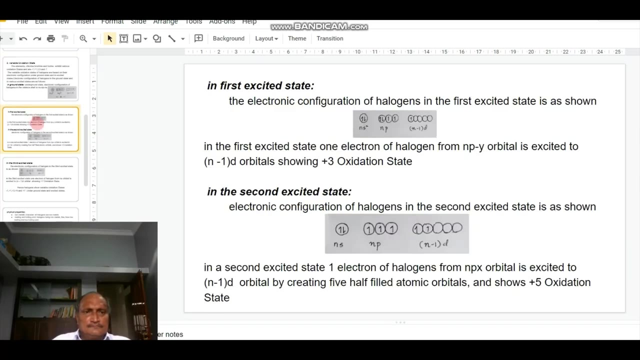 one electron and finally it becomes paired up, indicating an octave in the valence cell and it exhibits plus one and minus one as its oxidation state in the ground state, Coming to the first electron In the first excited state. the electronic configuration of halogen in the first excited. 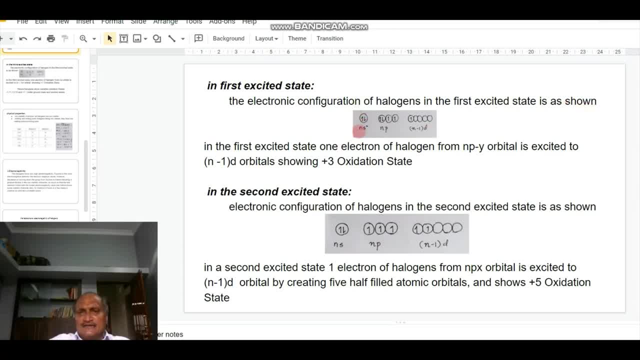 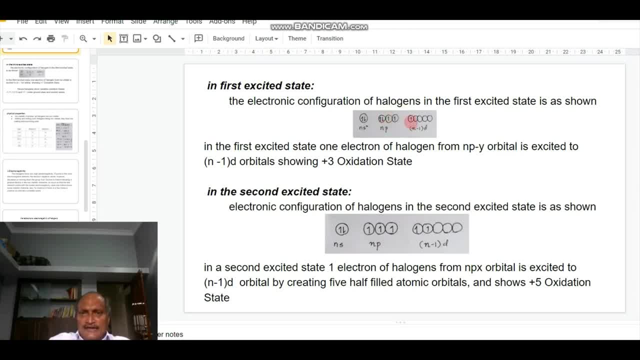 Here from the Npy orbital. Here from the Npy orbital An electron is excited to N-1d orbital. When an electron belonging to Npy is excited to N-1d orbital, here in the first excited state, the halogen exhibits three half-filled atomic orbitals. 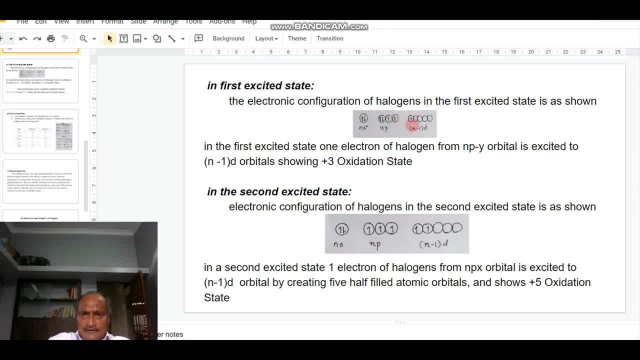 These are the three half-filled atomic orbitals. These are the three half-filled atomic orbitals. These are the three half-filled atomic orbitals Under the first excited state. Hence, the halogen in the first excited state exhibits an oxidation state of plus 3.. 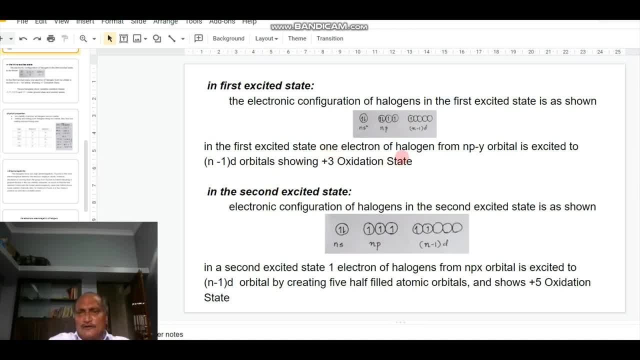 In the first excited state. one electron of halogen from Npy orbital is excited to N-1d orbital, showing plus 3 oxidation In the first excited state. one electron of halogen from Npy orbital is excited to N-1d. 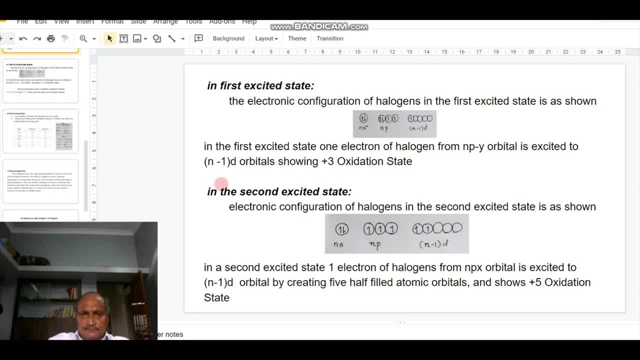 orbital showing plus 3 oxidation In the first excited state. one electron of halogen from Npy orbital is excited to N-1d orbital showing plus 3 oxidation In a second excited state, Here from the Npy orbital. 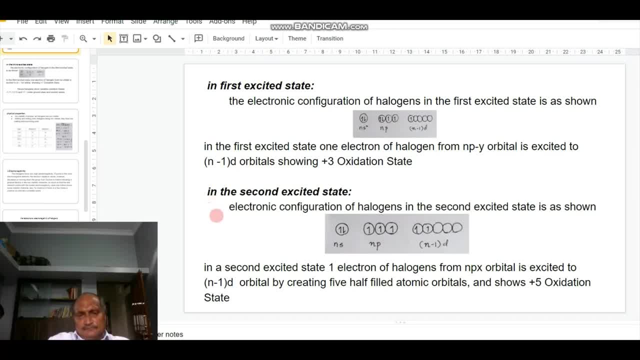 The next excited state is shown by Npy-1.. The second excited state is shown by Jys-1.. Here, the coming next electrical state is shown by J-1.. This figure is also the느 essentialת. This figure is thezubothering exercise, in fact, of the test. 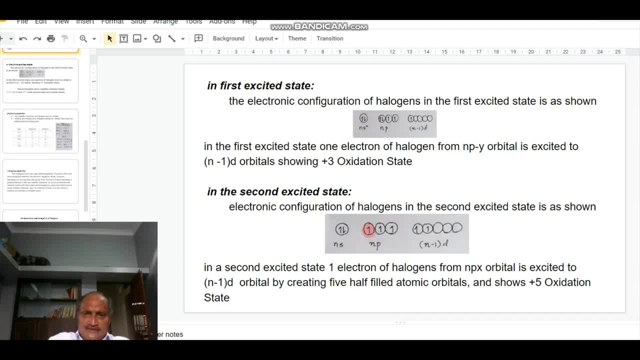 Be brave enough to study the next attacking states. Let's go on Now. let's look at the second cheated state Here, from the converge state is excited, to one more d orbital. Here, in the second excited state, totally, we are observing 5 half-filled atomic orbitals in halogens. These 5 half-filled atomic orbitals, 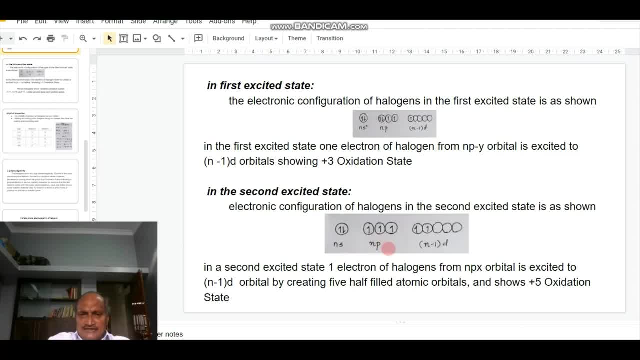 indicates the oxidation state of plus 5 for the halogens. So in the second excited state, one electron from halogen from npx orbital is excited to d orbital, thereby creating 5 half-filled atomic orbitals, and shows plus 5 as its oxidation state. The electronic configuration of halogens in the third excited state is as shown: ns1, npx1, npy1, npgy2, npg0, Z1 and N-1 d-orbitals are half-filled with one-one electron. totally there are three. 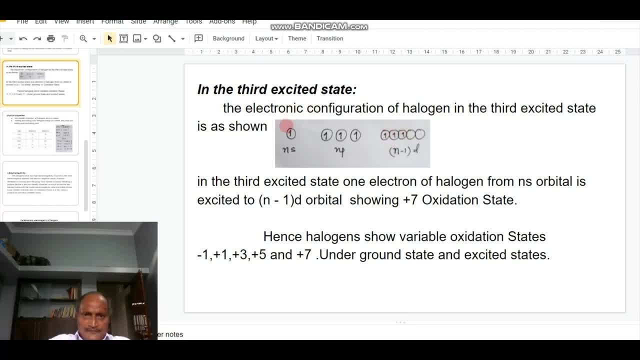 half-filled N-1 d-orbitals, Here, in the third excited state, one electron belonging to Ns orbital- Initially it is Ns2- in the ground state- and in the third excited state, the one electron belonging to Ns subshell is excited to N-1 d-orbital, thereby indicating seven half-filled 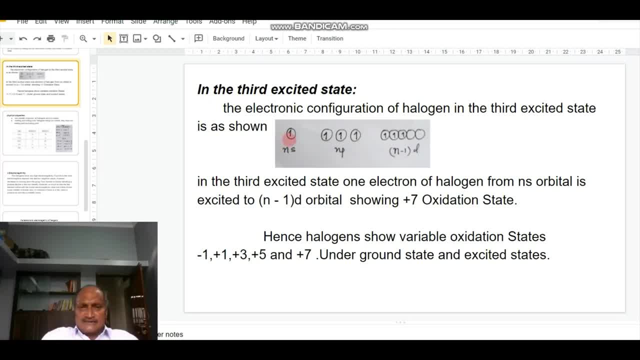 atomic orbital, That is one in Ns, three in Np and three in Ns And three in N-1 d subshells, indicating a total oxidation state of plus seven. So in the third excited state one electron of halogen from Ns orbital is excited to N-1. 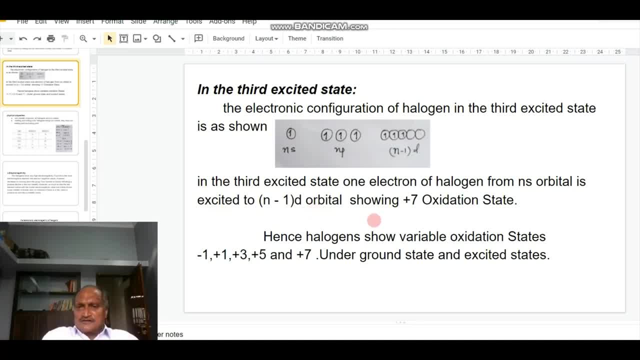 d-orbital showing three half-filled N-1 d-orbitals. Hence halogens show a variable oxidation state of minus one, plus one, plus three, plus five and plus seven in the ground state and in their various excited states. 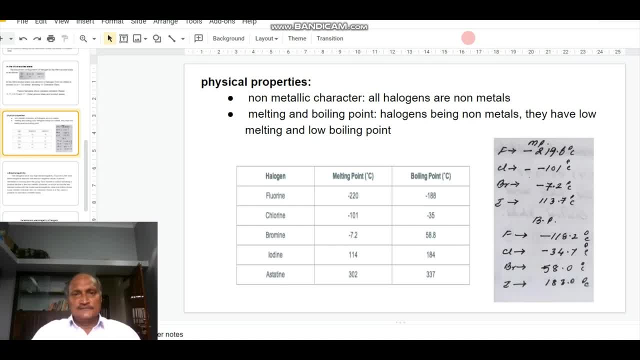 Coming to the physical properties of halogen, especially a non-metallic character. You know already about the properties of periodic or periodicity of the elements here, as we move from right to left in a periodic table, that is, from first A group to seventh A group, 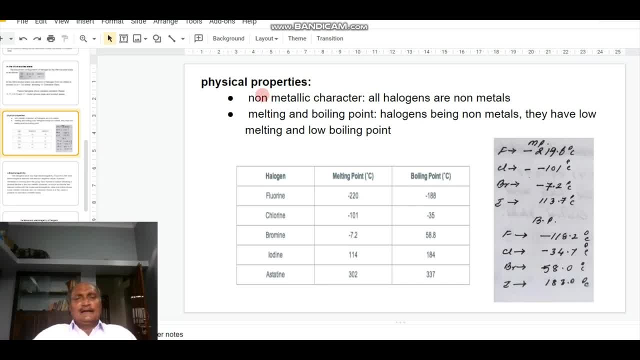 or noble gases. the metallic character will be goes on decreasing As we move from right to left in a period. the metallic properties will be goes on decreasing. Hence alkali metals are electrophositive metals, whereas halogens are electronegative. 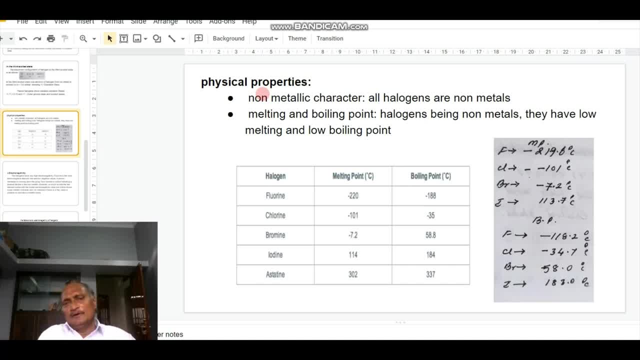 nonmetals. It means as we move from right to left in a periodic table, the metallic character will be goes on decreasing. Hence the seventh A group elements are nonmetals. Hence the seventh A group elements are nonmetals. 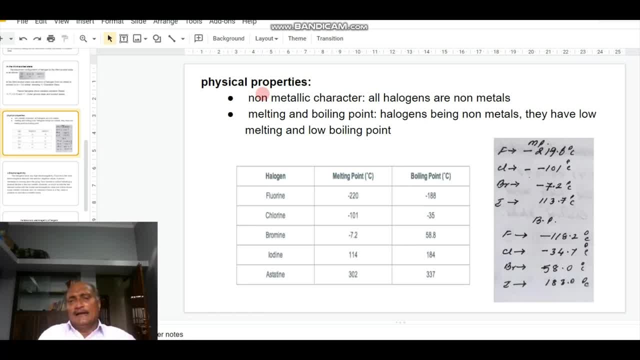 Hence the seventh A group elements are nonmetals. Hence the seventh A group elements are not. Hence the seventh A group elements are nonmetals. However, as we move from top to bottom in a group in the periodic table, in any group, 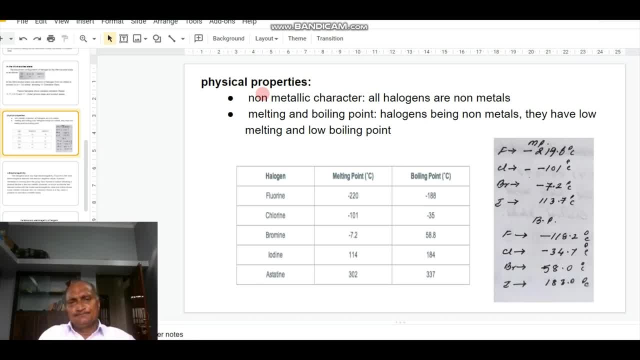 that is, as we move from top to bottom in any group in a periodic table, the metallic character will be goes on increasing. It means the first member of the halogen is a non-metal, highly electronegative non-metal. As we move from fluorine to chlorine, chlorine is again a highly electronegative non-metal. 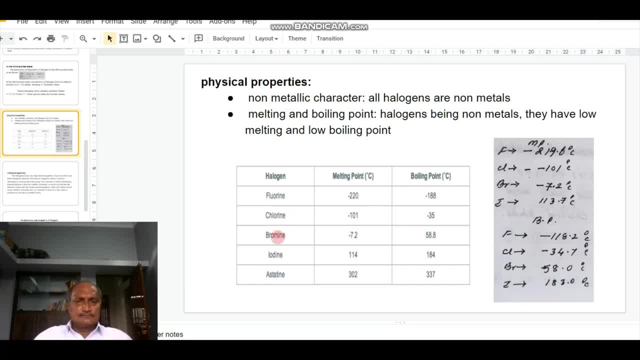 As we move from chlorine to bromine, bromine is also a non-metal. When coming to the iodine, iodine is having an electropositive character and it shows a metallic nature. It means, As we move from fluorine to chlorine, chlorine to bromine, bromine to iodine, the electronegativity. 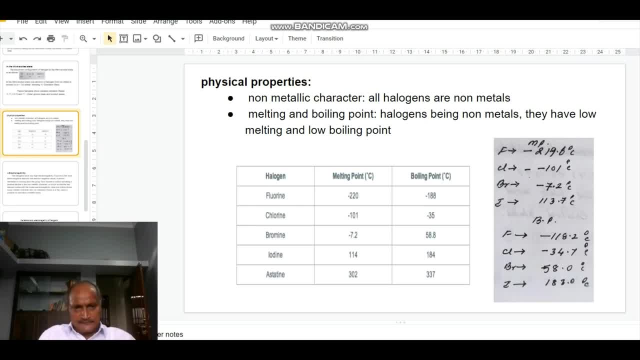 character will be goes on decreasing. It means electronegativity decreases means, similarly, there is an increase in the electropositive character. Hence Fluorine is highly electronegative- the first member of the family- and iodine is electropositive. 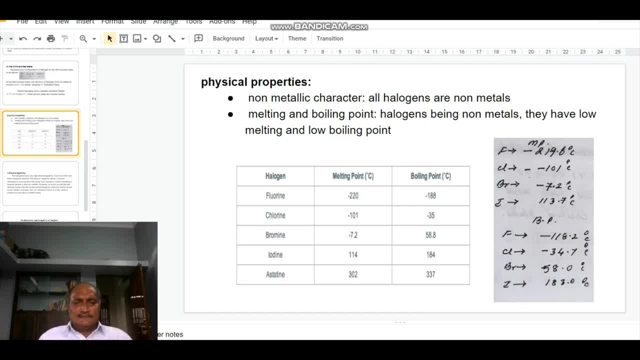 and it is a metal. So here, as we move from top to bottom, the metallic character increases. hence iodine is exhibits, a some of the metallic character. Hence The next property is electronegativity. looks like a force and it forms many of the complexes. 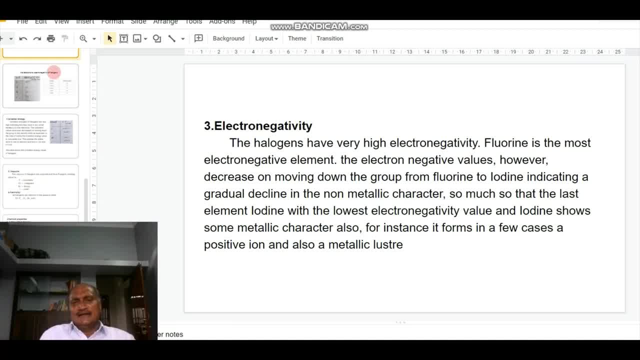 Coming to the next property, that is, Electronegativity. as we know, halogens are highly electronegative in nature, So we Fluorine is the most electronegative element. The electronegative character or the values of electronegativity, however, decreases on. 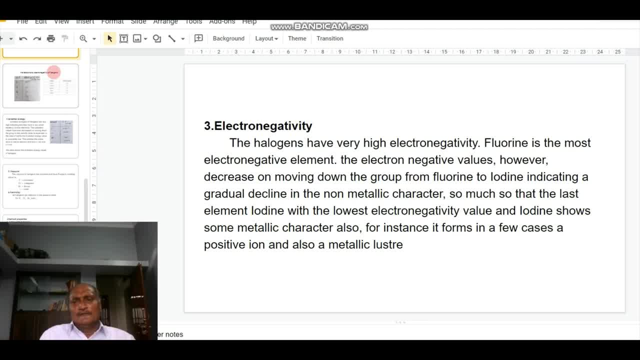 moving down the group from fluorine to iodine, indicating a gradual decline in the nonmetallic character. so much so that the last element, iodine, with the lowest electronegativity value and shows a sum of the metallic character. 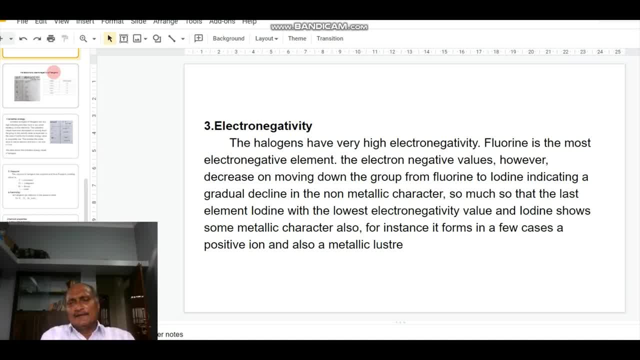 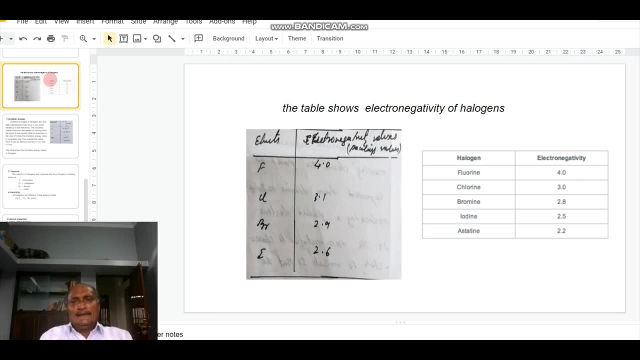 Also, for instance, iodine forms in a few cases a positive ion and also a metallic luster. Thank you. The table indicates the electronegativity values of halogens. The electronegativity of fluorine is 4.0, chlorine is 3.0, that of bromine is 2.8, iodine. 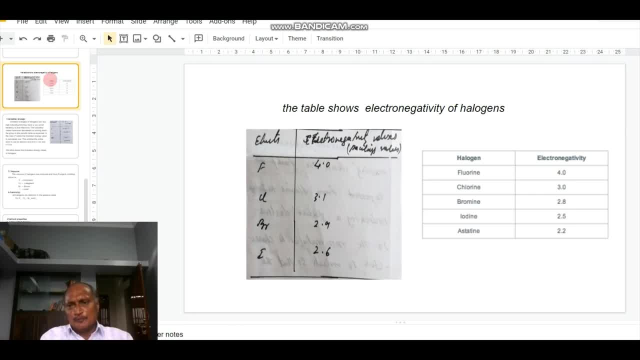 is 2.5, and astatine is 2.2.. The table clearly shows that As we move from top to bottom in a group, electronegativity character will goes on decreasing. Hence fluorine is having a highest electronegativity values of 4.0, and iodine is less electronegativity. 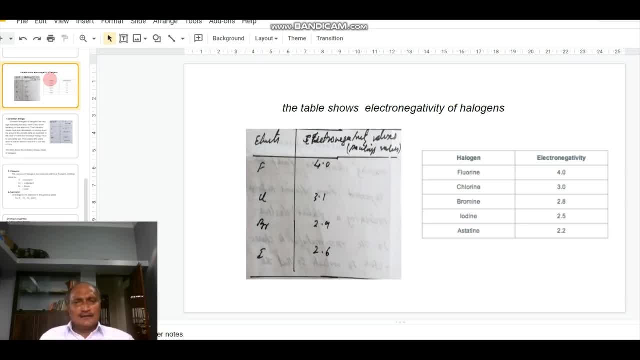 value having 2.6.. Here the electronegativity values are measured in terms of electronegativity. Now let's look at an example of fluorine. Here, fluorine is having a highest electronegativity value of 4.0, and iodine is less electronegativity. 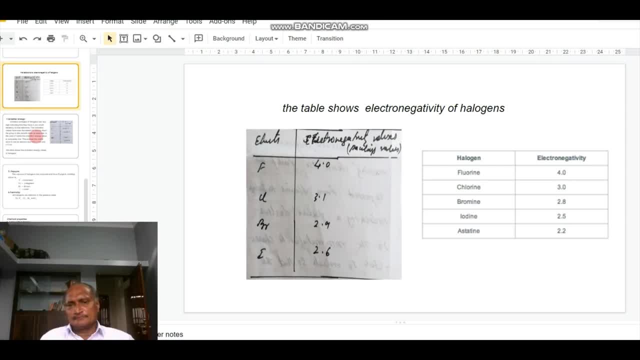 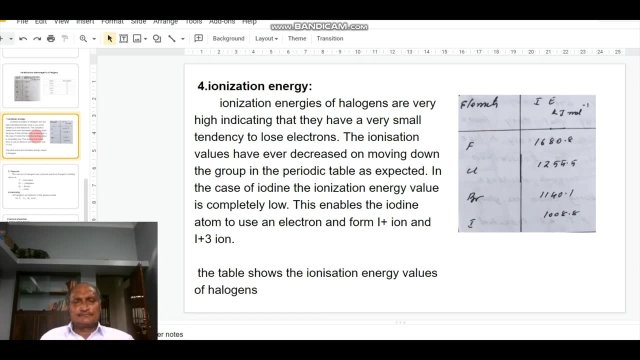 value, having 2.6.. And now let's look at a pollens scale. coming to the ionization energy, From our previous discussion we came to know that ionization energy is nothing but the amount of energy required. This is the unit of energy. 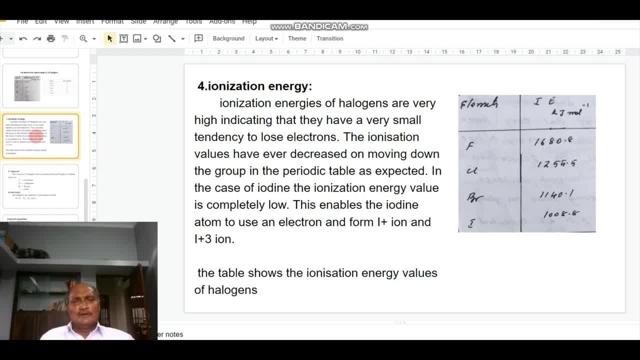 The unit of energy is working rate, So that's why this is not financially beneficial. to remove an electron from an isolated gaseous atom while converting it into its cation is called as ionization energy, and ionization energy is indicated by Ie or Ip. 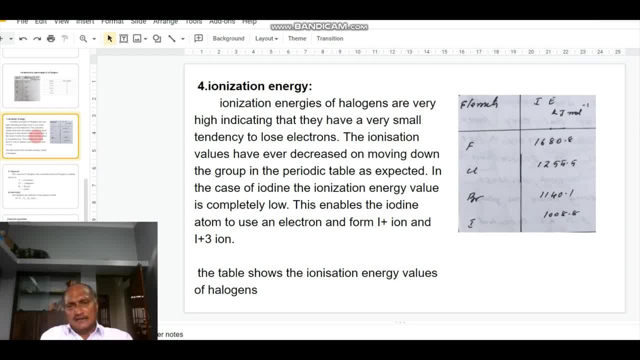 Ionization energy or ionization potential. So here the ionization energies of halogens are very high, indicating that they have a very small tendency to lose electrons. The ionization values, however, decreases on moving down the group In the periodic table. as expected in case of iodine, the ionization energy value is 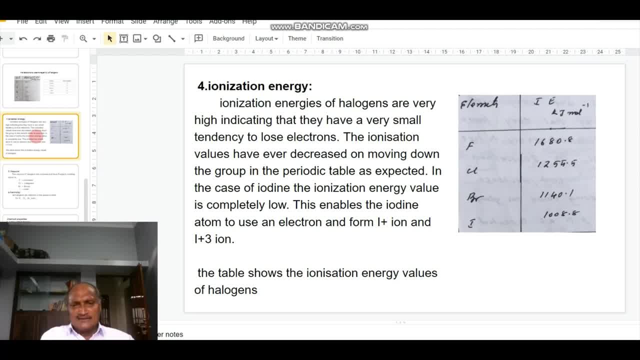 completely low. This enables iodine atom to use an electron and form plus one ion, and it forms plus three ions. So here the ionization energy values of halogens are very high. They are measured in terms of kilojoules per mole. 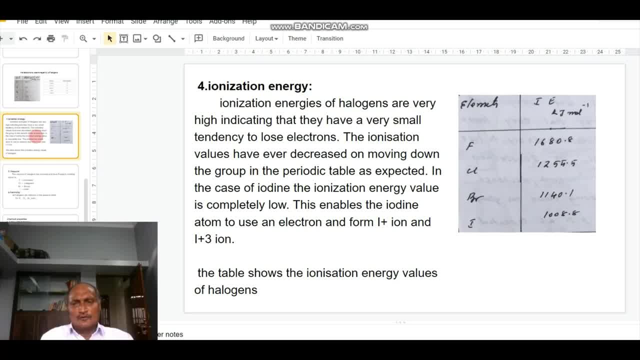 So fluorine is having a highest electronegativity- sorry, highest ionization energy values of 1680,, that of chlorine is 1255,, bromine is 1140, and iodine is 1008.. The table shows the ionization energy values of halogens. 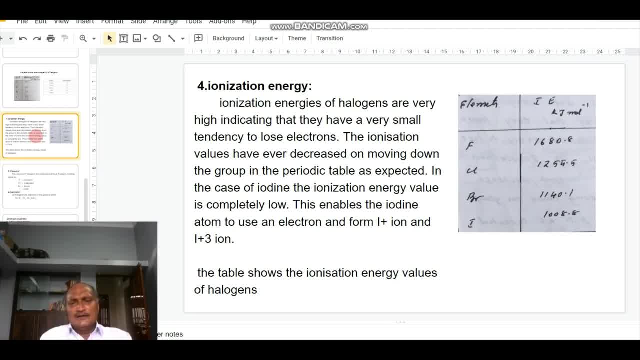 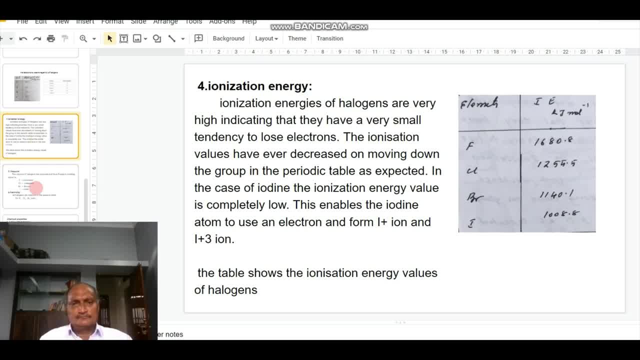 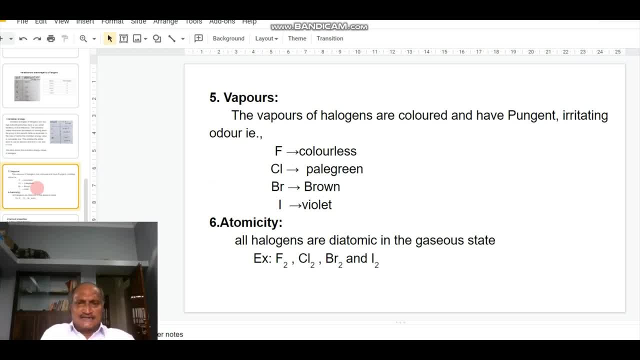 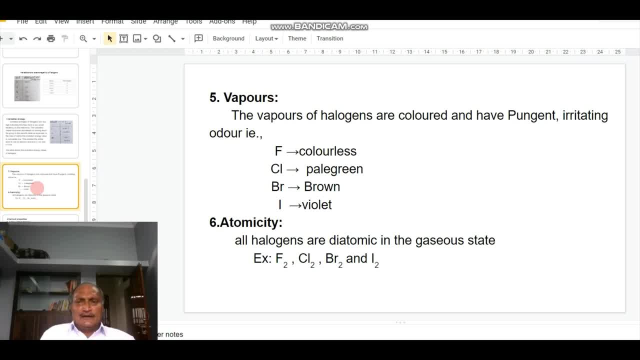 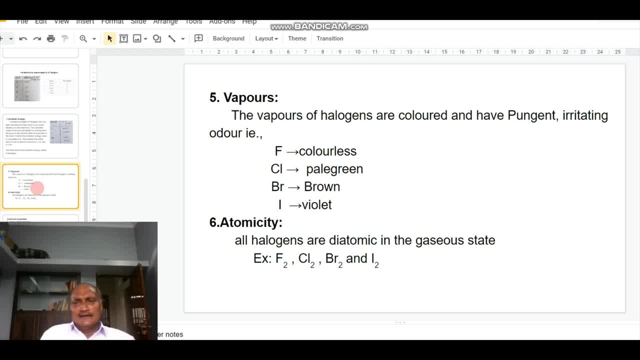 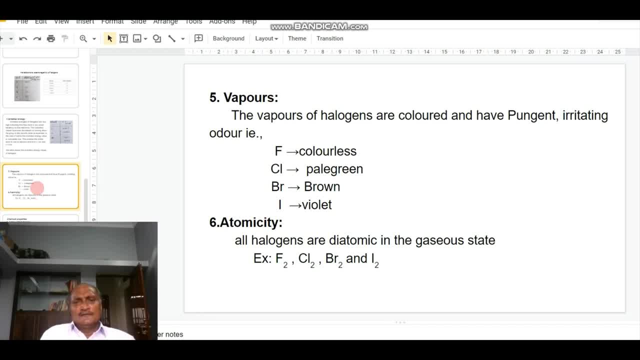 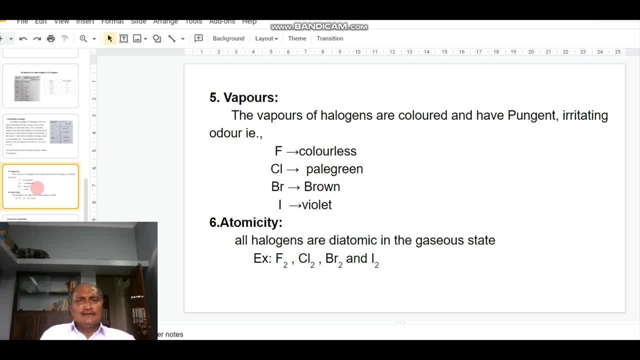 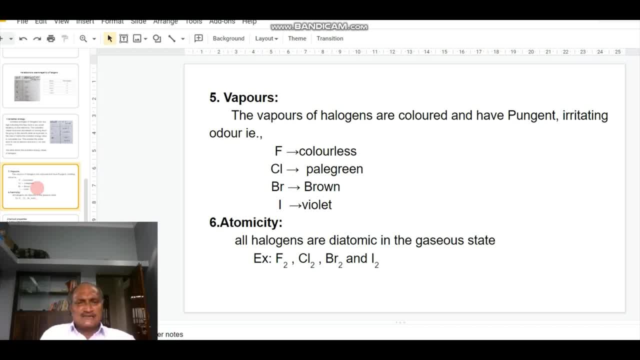 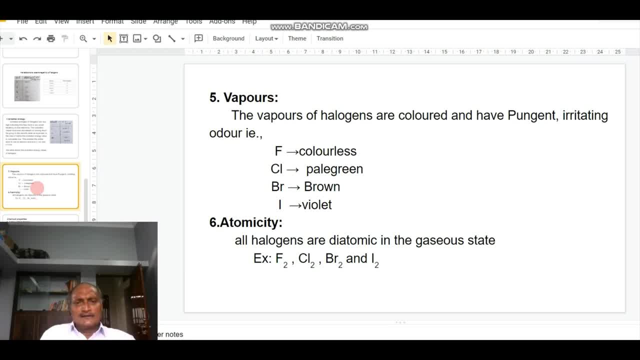 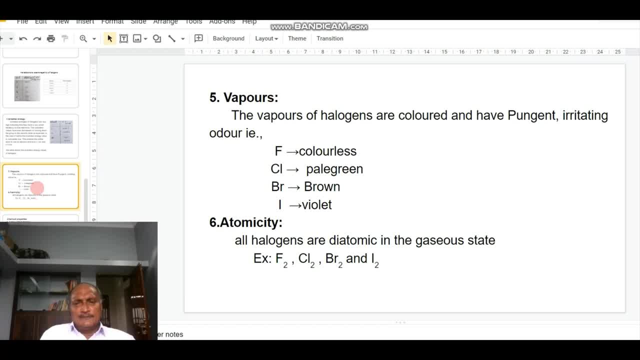 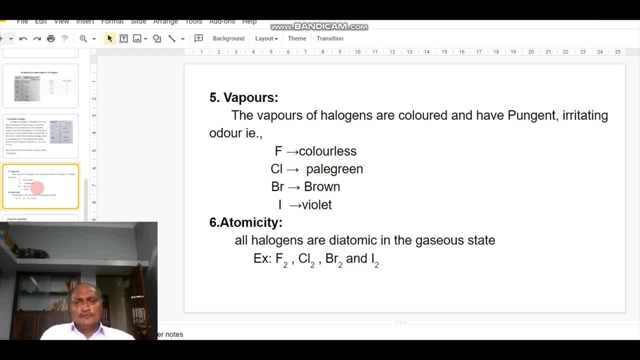